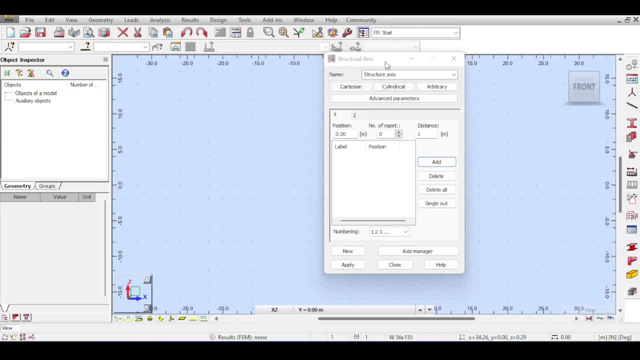 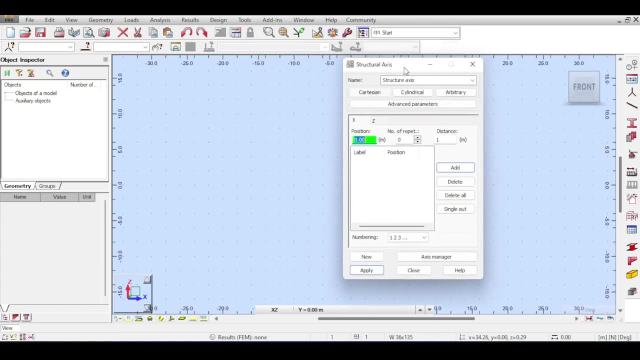 here, which will be covered in a separate video. In this video we are just trying to draw a beam, as simple as possible, without a lot of details. There will be a separate video about grids and how to use them or structural axes in the future. Now, in the beam that I have here, I want to draw a 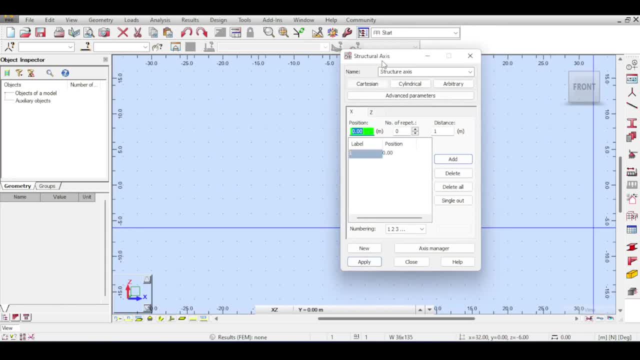 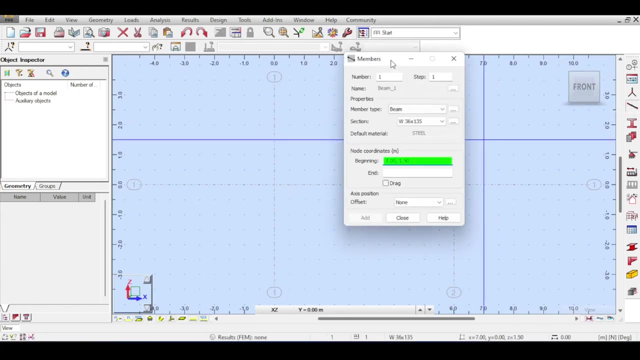 beam that is between x equals zero to x equals six. The z is basically zero. There is only one z. I will apply and close and you can see we have two grid points. Now to draw the beam. we simply click on members, which will open the member drawing. 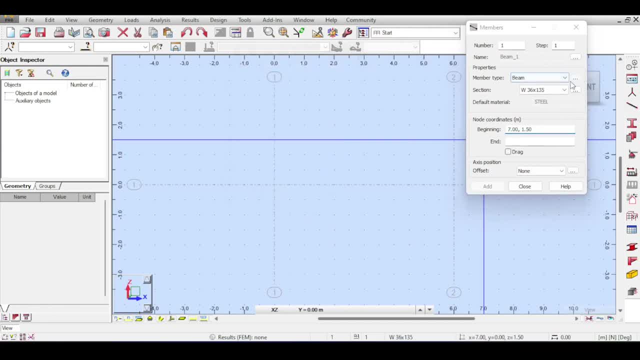 system. The member type is a beam. There are various types that we will talk about later. Now we'll just keep the beam. The section here is some sort of steel section which we don't want, So we'll click on that to browse the sections and define our own sections. You see, if the section 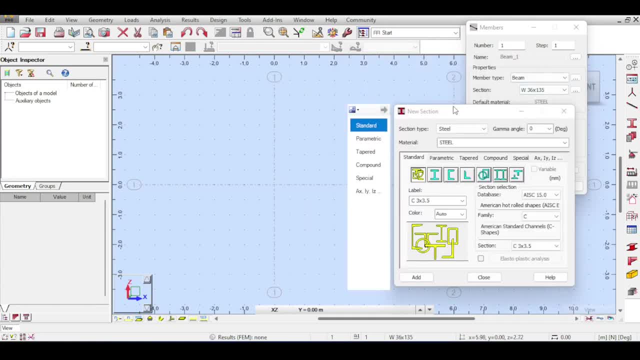 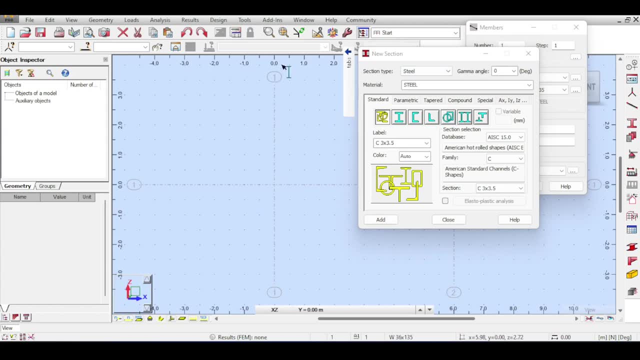 you want is not here. you can click on that and you will see that the section you want is not here. You can browse and select your own section. Now let's say that the section is a 300 by 500 millimeter reinforced concrete section. Now, as you can see, the sections here are steel compatible and I 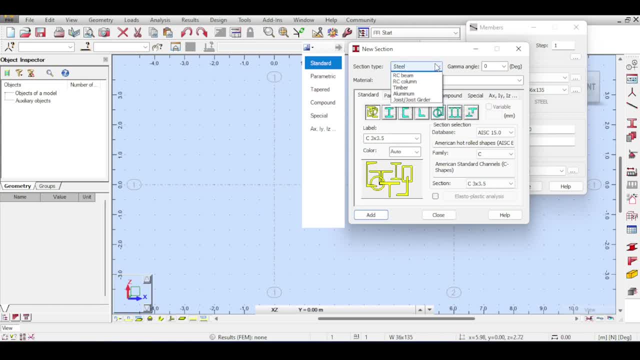 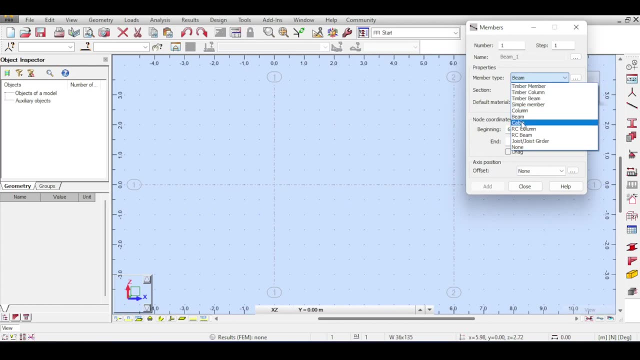 don't see any concrete type. Now the reason is because the section type is steel. Now if you select a reinforced concrete beam section type, it will switch to reinforced concrete friendly sections. This can also be done by clicking on the beam here and instead of selecting a general beam, 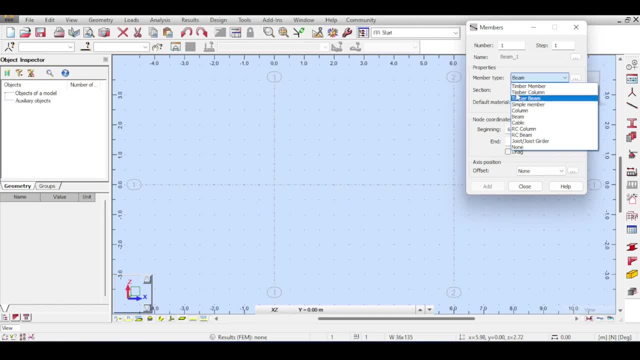 you can select a reinforced concrete beam. The other types are going to be subject for other videos. Now, if you select the reinforced concrete beam and now select the sections, you can see sections that somehow make sense. but if you don't find your section, you can click on the browse and 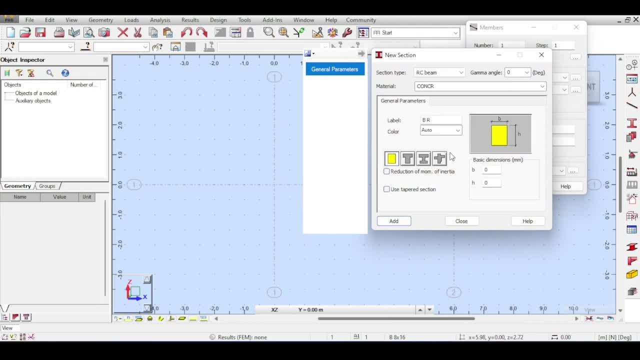 you can see that it immediately opens reinforced concrete friendly sections. Now we want our section to be 300 in width and 500 in height, so let's type that. You can choose to use tapered sections or use the same section, and we will get a similar result. And now let's start discussing our project. 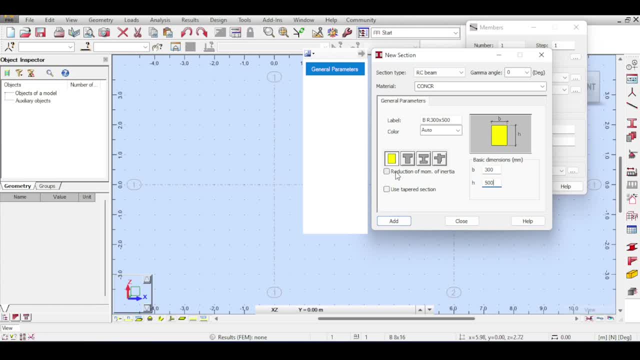 So let's first start with the project. So let's say that we have a section called the reduction of moment of inertia- Those, at least the reduction of moment of inertia has an application, especially in design codes, in the ACI code. but this is something that we will do later, when we start. 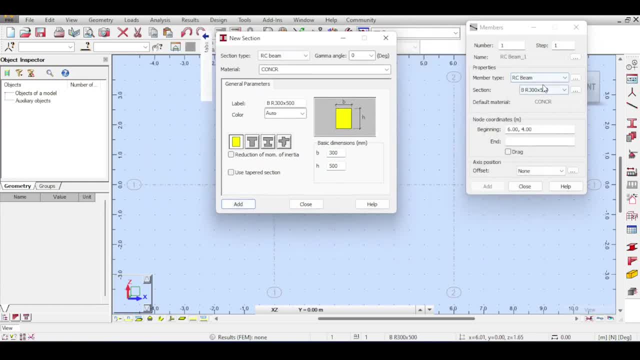 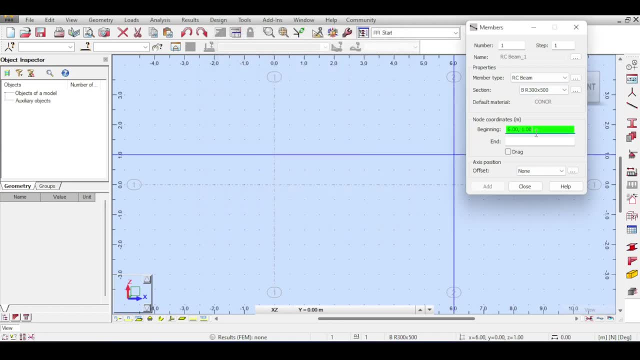 discussing real projects. For now, this is a tutorial, just to get things rolling. so let's keep those settings as they are and let's add the section Now. strangely, you think the section was: there is a beginning, there is an end. well, you take your cursor, you can see. 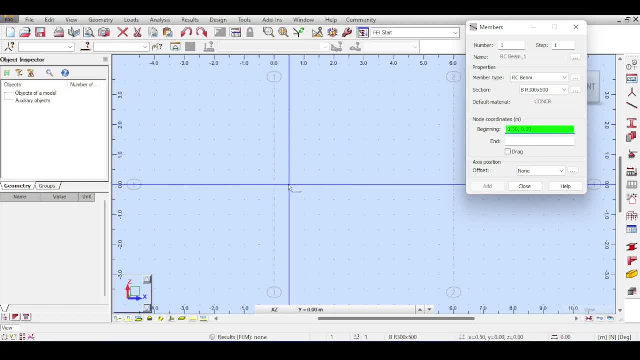 that it's floating around and you can see that when you are approaching the grid point, there is a diamond, meaning that it's snapped to the grid. you can also see that the cursor is actually snapping to the drawing, so you were perfectly able to draw a beam without a grid. however, having a grid is good. 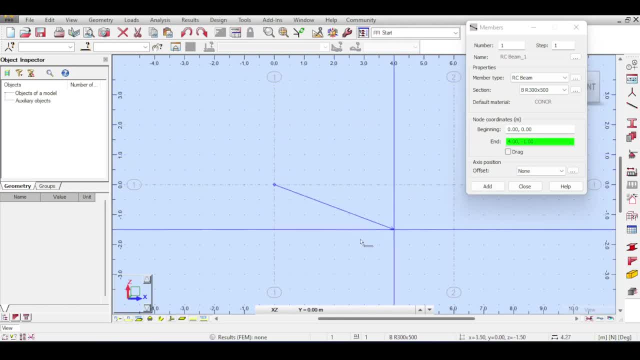 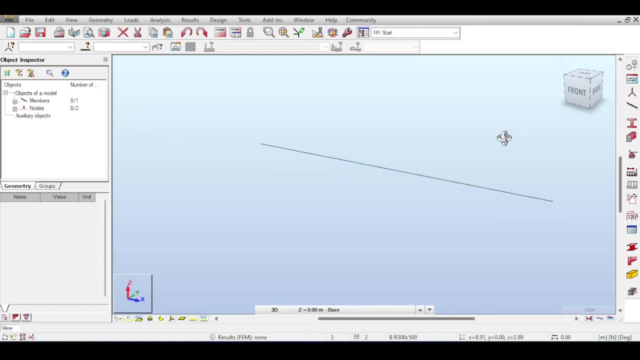 practice and that's what we're gonna do. so you click on the start, you can see I'm dragging the beam with me. you click on the end and you have your beam. now you can basically go to an isometric view if you want, if you find yourself in. 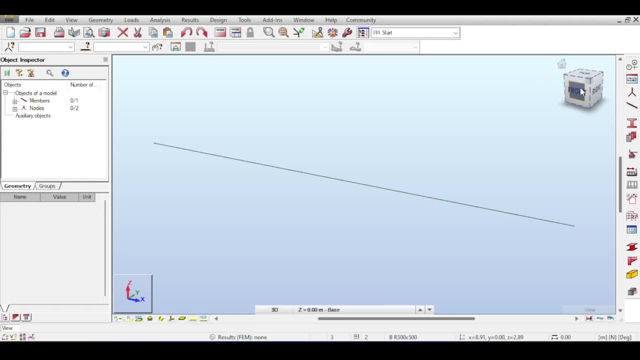 the isometric view and want to go back to the front of you. you can click on front, but it doesn't seem to be right, like where are the grid points? so if you double click on front, you will get back the grid points. as you can see, I'm gonna. 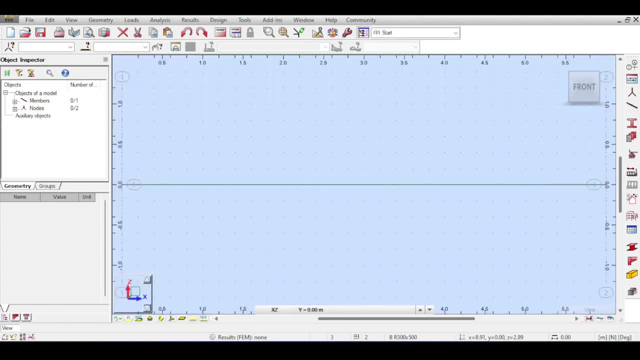 go to the isometric view. now we need to apply supports. the only supports I support I had was a fixed support at a, and by the way, you can see that my cursor was somehow behaving strangely. it was this me, which means I can no longer select. so if you move, you cannot select anything. 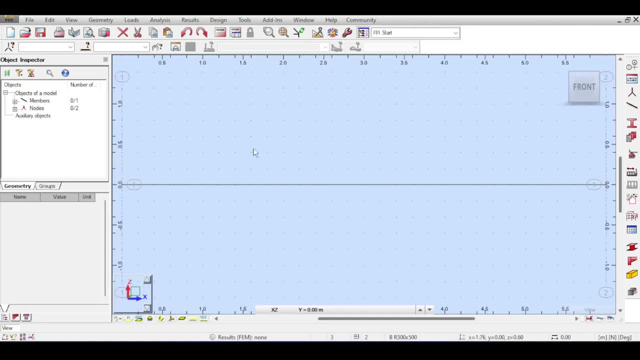 now to get rid of this problem, you can right-click and say cancel, which gives you back your original cursor that you can select and pan with. now, panning is done by the middle button of the mouse and zooming in and out is done by moving the wheel of the mouse. okay, so we want to have a fixed support here. so what do? 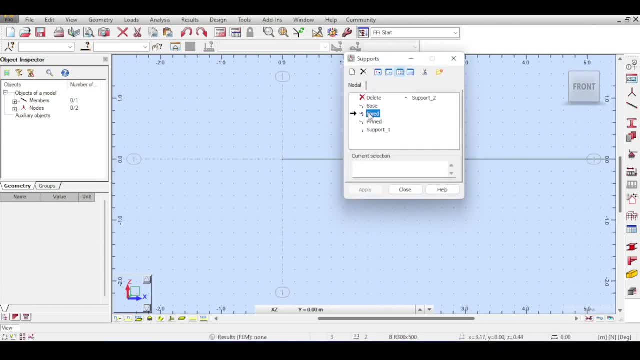 we do? we go to supports. there is a fixed support here. we click on it and click on the bundle node. sometimes if you click on the node, that doesn't apply. well, if it doesn't apply, like this, if you click on the node and doesn't apply, 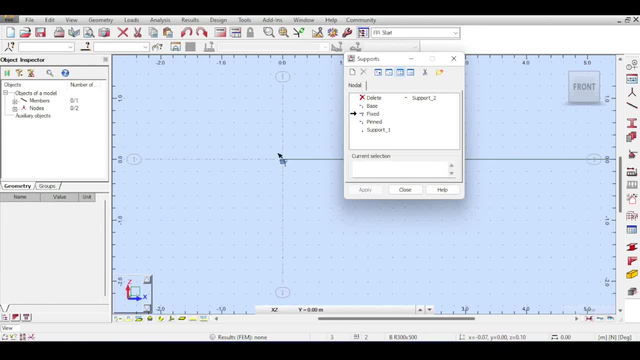 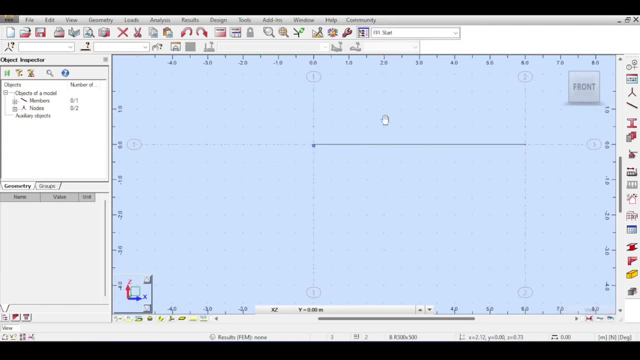 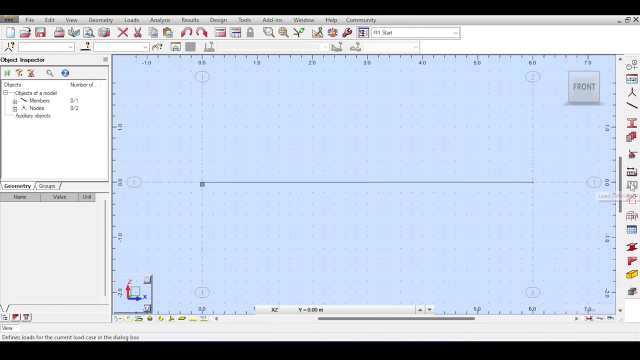 then you simply click on apply and it will apply, basically, and this is the fixed support. now, it's very small and there is a solution for this support being so small. however, I will leave it as it is because this is an initial tutorial, so I have my support. now let's go back to our loads. so if you want to, 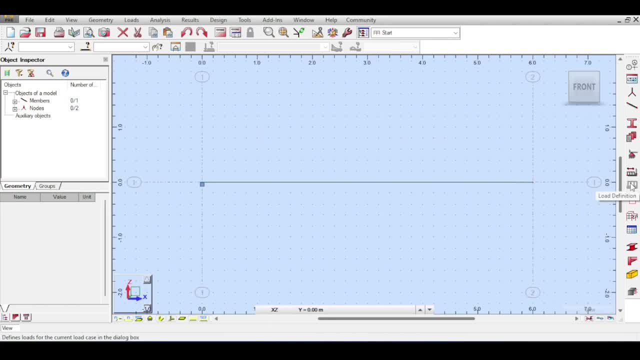 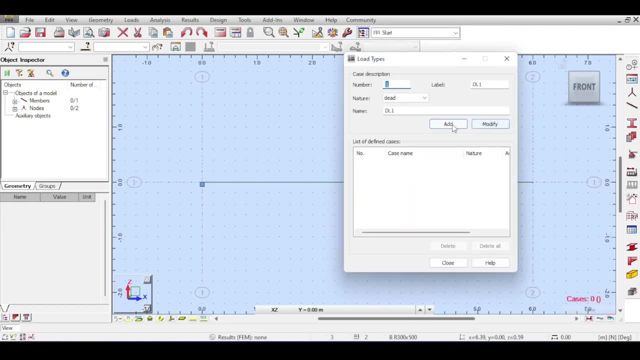 add loads. as you can see here, it's grayed out. the reason why it's grayed out is because there are no load cases or types defined, so you click on load types, add the load case and then close it. so now you can apply load definitions. there will be more tutorials covering load. 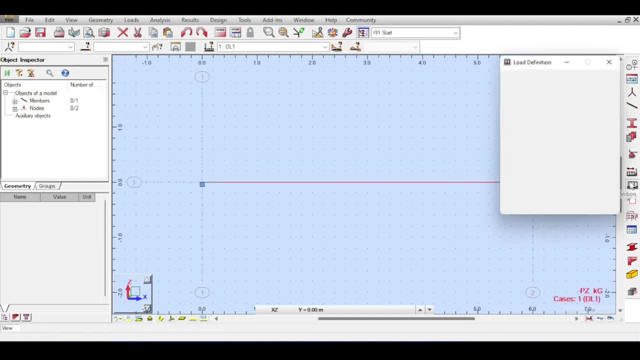 cases. however, this is a very quick example. so, going to the load definition, you want some loads, so we have a member load which is a load on a beam. we want a trapezoidal load that is between two points in the z-axis- the initial load. 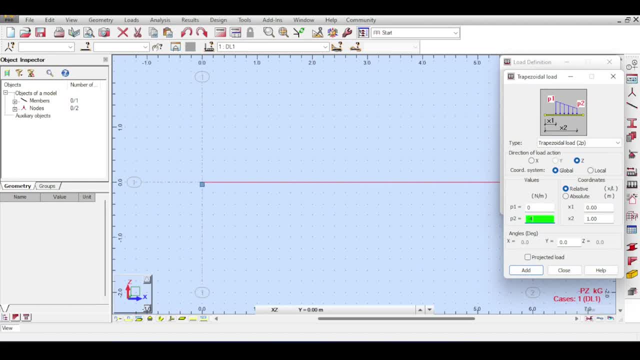 was zero and the final load was negative. four: it was applied in the z-direction down and it was applied between x equals zero and x equals three. please notice, you want to use the absolute because we are taking distances. so that's it add. we go now to the beam. we click on the start. 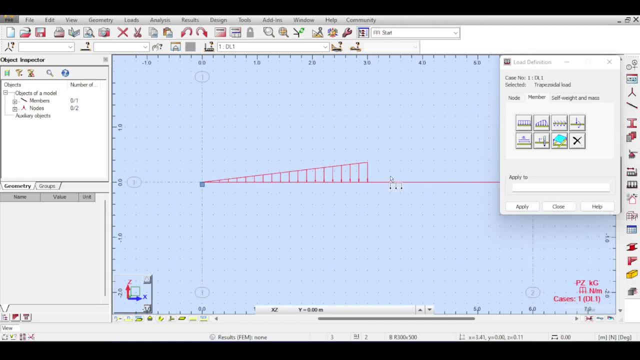 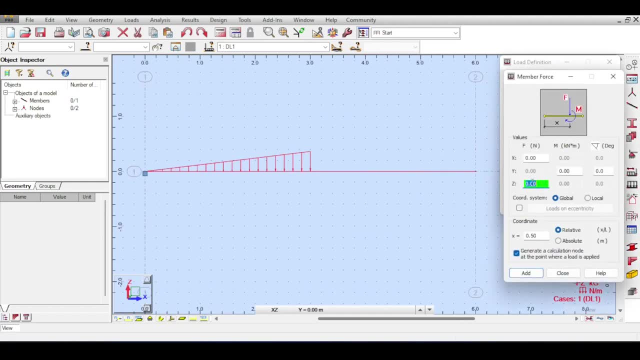 when you click on it you have the first load. now we want another load which is the two kilonewton at 1.5. so we choose this load member force. we say it's a negative 1.5 kilonewtons going down to negative 1.5 kilonewtons going down to. 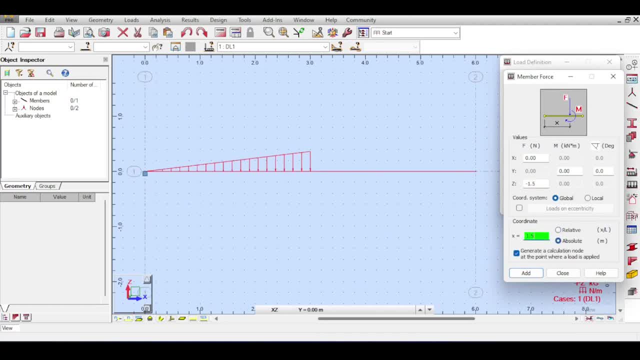 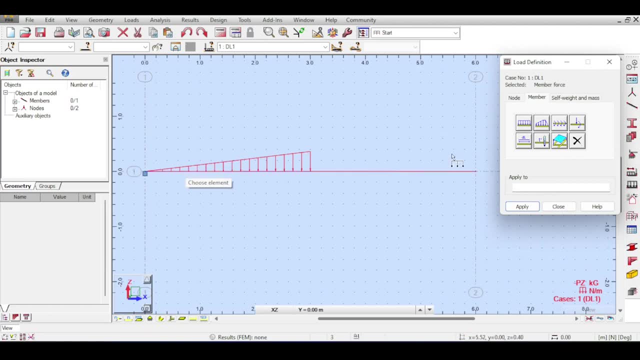 negative 1.5 kilonewtons going down to negative 15 kilonewtons- going down, it's once again- and absolute distance of 1.5. now, if you click here, this would be a mistake because you would measure 1.5 from the left side. so what do we do? we go. 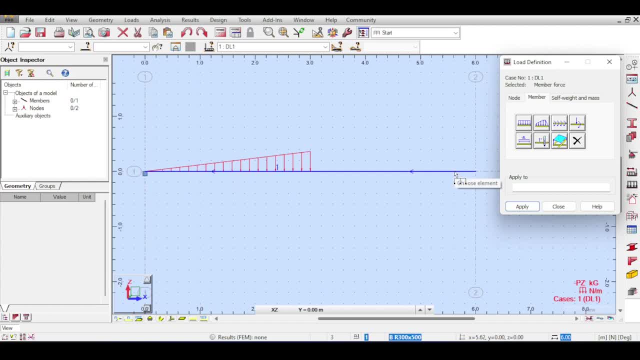 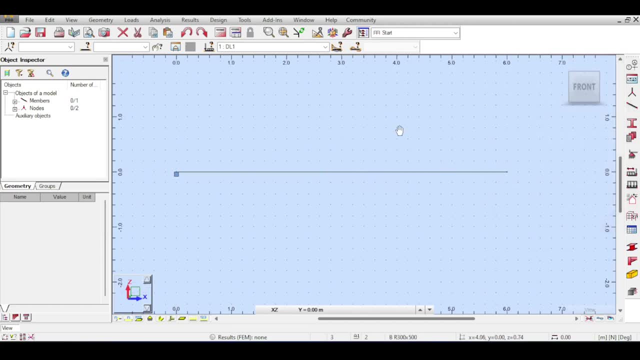 to the right side to indicate to robot that we are going to measure our distances from the right side. if you click on that, you have your force and that is basically it. now, if you close, you realize that the forces gone missing. now, did we lose our forces? well, no, the robot tries to basically show you what. 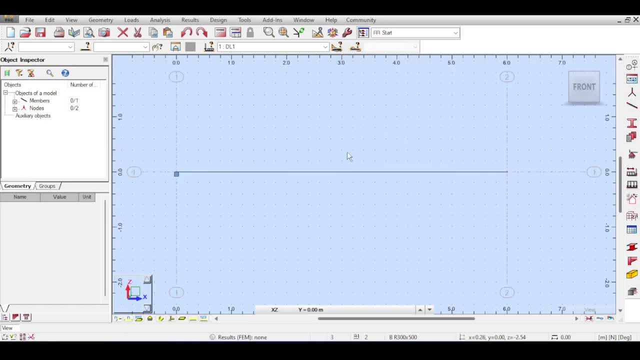 need it. So all you have to do if you want to see the forces all the time is to go to the display settings. You can see that there is this little icon with load. If you click on it, you see the loads. If you click on the label, you will see the values of this load. Now let's just run the. 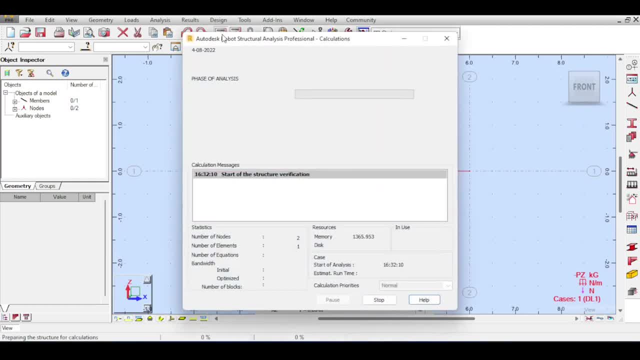 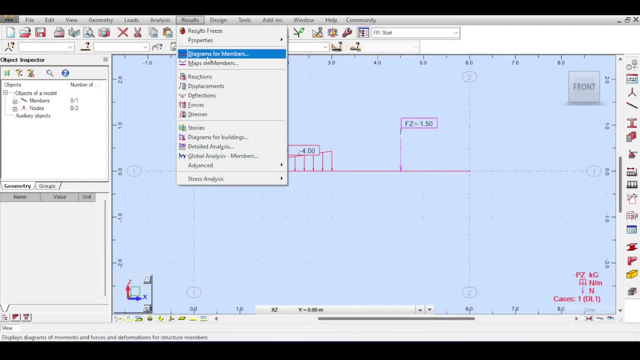 analysis. We will click on this calculation tool which will run the analysis. Now, there are no mistakes in our model. It ran the analysis. You can open the results and just choose the diagrams from EMBARS. Say, for example, MY, which is the bending moment in Y. You can hide the loads.